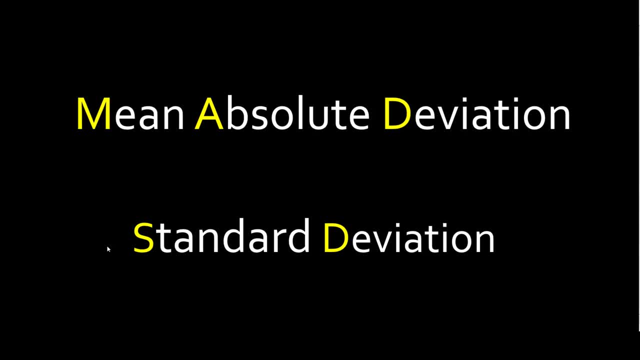 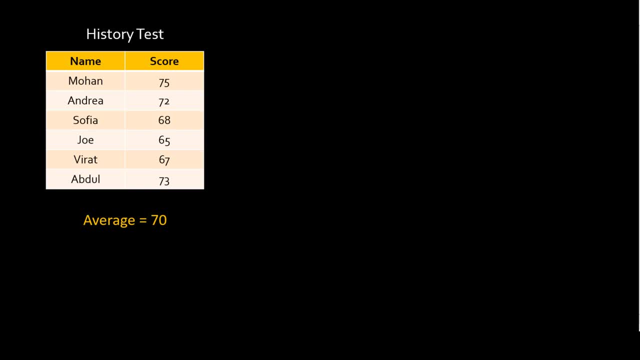 In this quick video we will learn what is mean absolute deviation and standard deviation. Let's say you have a history test scores Here I have six data points where I have shown the scores out of 100 and the average score here is 70. And when you plot this on a chart, you will 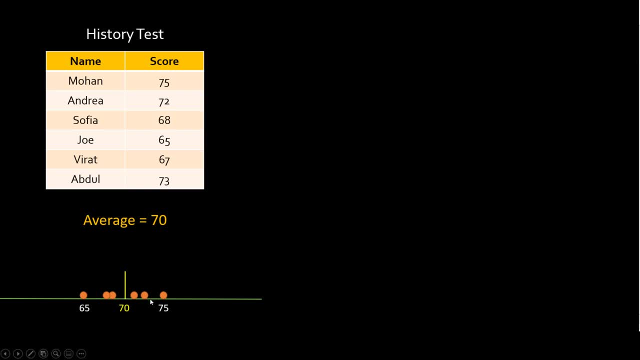 see that 70 is an average, this yellow line and these are the individual data points. For example, you have 75 here, you have 65 here, and so on, And you can see that all these data points are near the average data point. So what we're trying to learn is how far apart the individual data 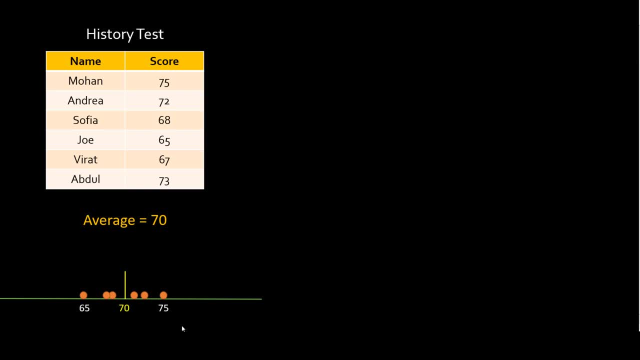 points are from the average, or how spread out the data points are with respect to average. You can have a different data set. let's say a data set of a particular data point, and you can have a different data set. let's say, a data set of a particular data point and you can have a different data set. let's say 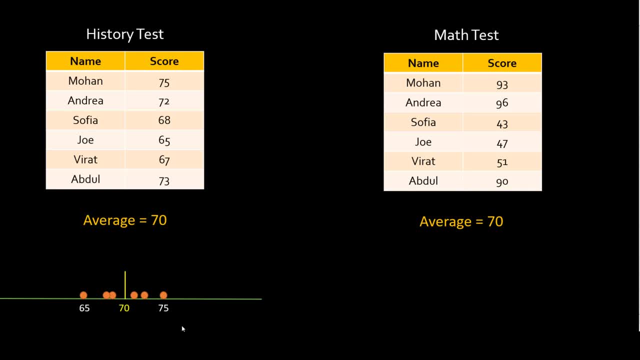 a score in a mathematics test and those scores might look like this: Again, the average is same, but when you plot them on a chart you will find that data points are quite spread out. They are quite far away from average data points And in statistics and data science it helps if you can. 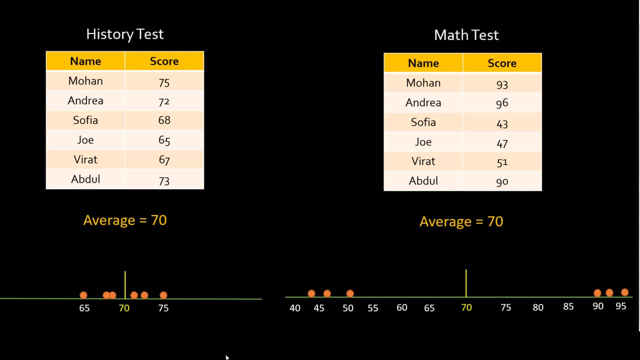 figure out how far apart individual data points are from the average data point or how spread out these data points are, And we need a metric or a number to represent this concept Here. my data set is simple. I can easily say that in the right hand side the data points are far apart, But when you 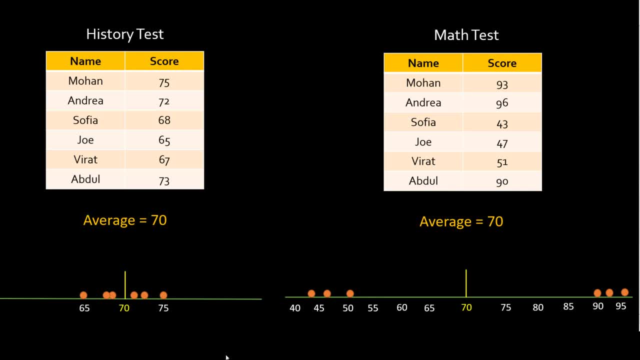 have millions of data points, and if you want to come up with a single number or a metric which can tell you this, then that will be super useful. So pause this video for a moment and think about what that metric is, And if you want to come up with a single number or a metric which can tell 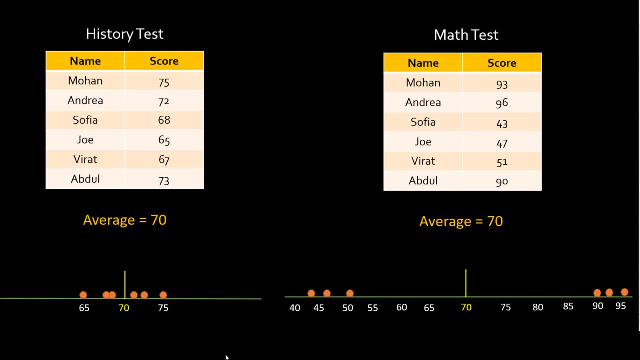 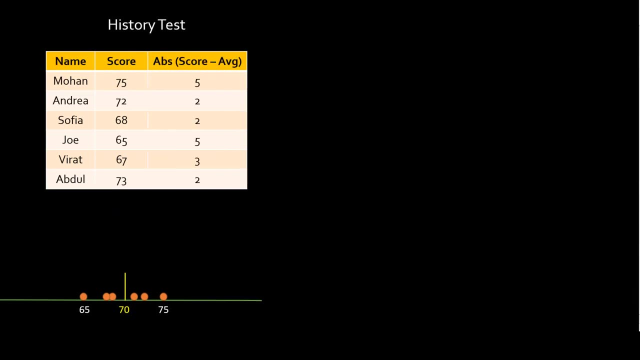 you this, then that will be super useful. So pause this video for a moment and think about what that metric could be. Well, a very basic approach, common sense approach, would tell you that. why don't you take the difference of individual score with respect to average? So let's do that: 75.. How far away it is. 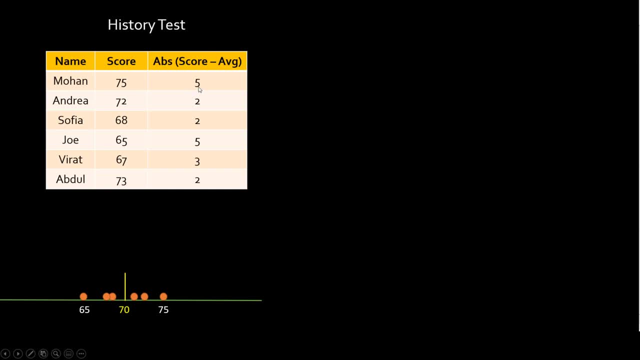 from average. Well, my average is 70. So this guy is five points away. Similarly, 72 is two points away, 60 point is 68 is two points away, and so on. And if you take a mean of this number, that will be three point one, six. And for the second case you do the same thing. and when you 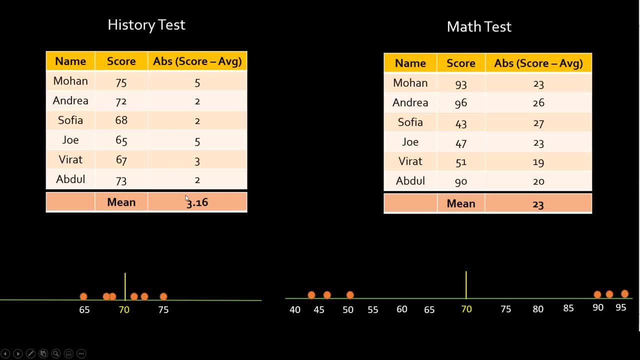 take a mean, you get 23.. So now this is interesting. Look, this number is telling you that for the history test my mean is three point one six, But for mathematic test my mean is 23.. Which means, if here I have a higher number, And that implies that this particular data set the mathematic test, that 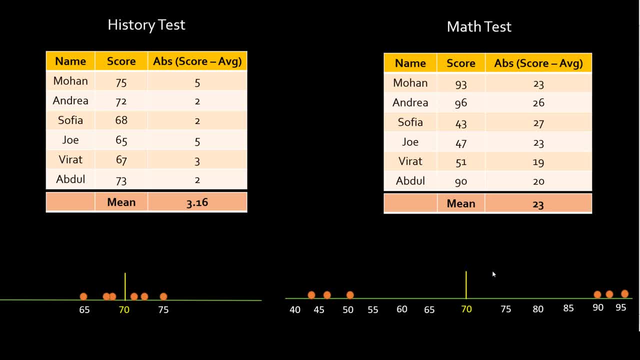 I said is widespread out, you know, with respect to the average number. So this is interesting. Now, this mean number is nothing but mean absolute deviation. You can also call it mad, MAD, Alright, So MAD Could be quite significant, or a unique number. 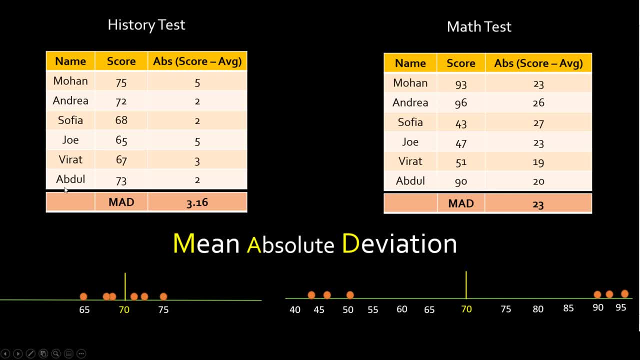 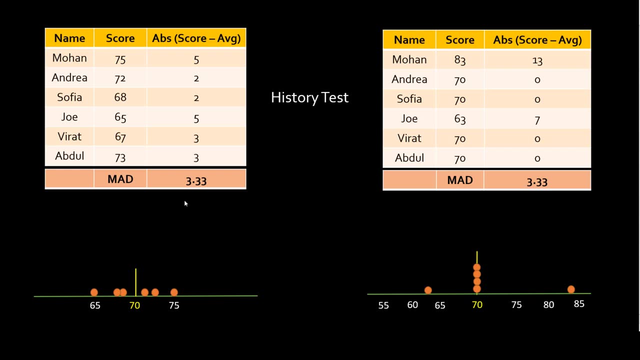 useful metric that can represent how spread your data points are. but there could be a scenario where using mean absolute deviation might not be enough. Let's take this particular example here. see here: mean absolute deviation is 3.33 on left and right hand side. but if you look at the chart, 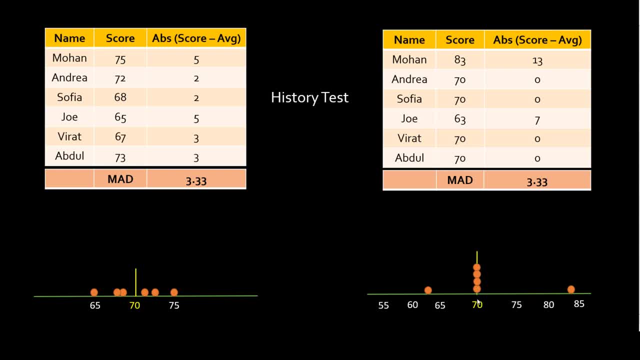 you can see that on a right hand side, although I have four points right at the average, but I have one data point which is far away. see, this is far away. on the left hand side, all my data points are between 65 to 75 range, but here my data points are in 63 to 83 range, so my range is widespread. 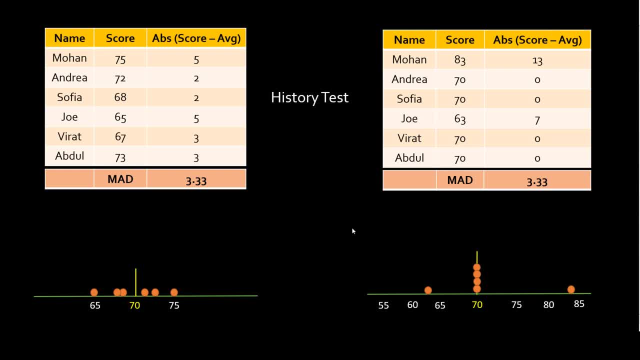 so here the data distribution is kind of spread out and when you look at the chart, at MAD, it tells you it's the same number, 3.33. so in this case MAD is not very useful, so we need to come up with something else. again, pause the video. can you come up with? 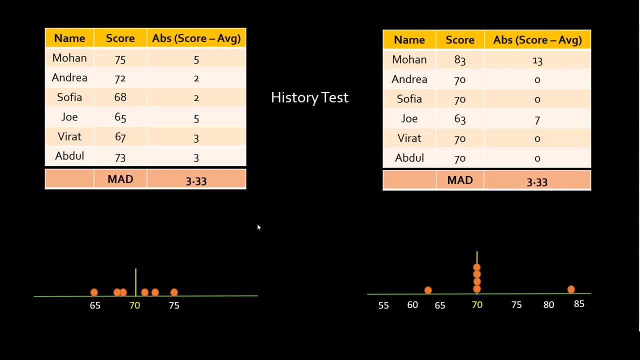 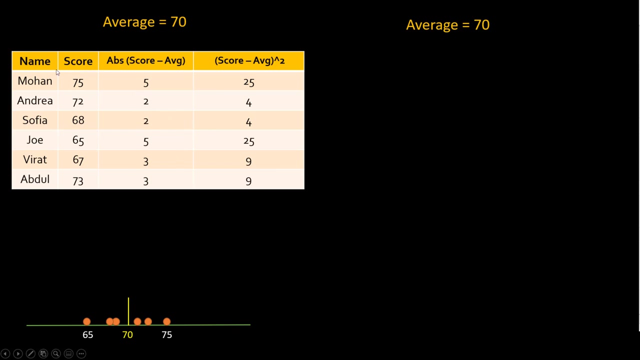 some other concept which can represent this data distribution accurately. well, if you give it a little try, you might come up with this idea that how about we again, we keep the same data set, same absolute everything, but we add a new column and we take a square of these individual numbers. so here see, look at this column. 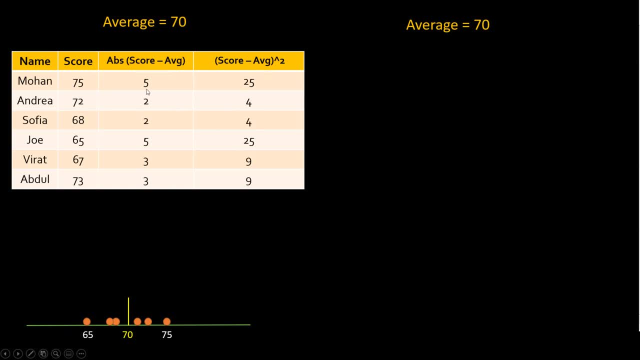 this column is nothing but the square of this second column. so 5 square is 25, 2 square is 4, 2 square is 4, 5 square is 25 and so on, and then you take an average of this column. okay, I took. 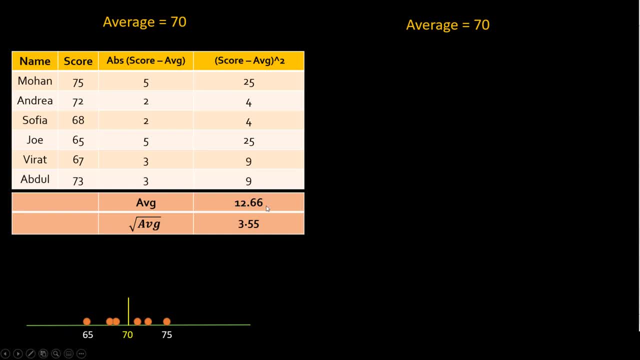 the average of this column, which is 12.66. then I took the square root of that average. why did it take square root? well, because you square the numbers here and usually, therefore, you want to do a square root. okay, so here I come up with number 3.55, on the right hand side. I do the 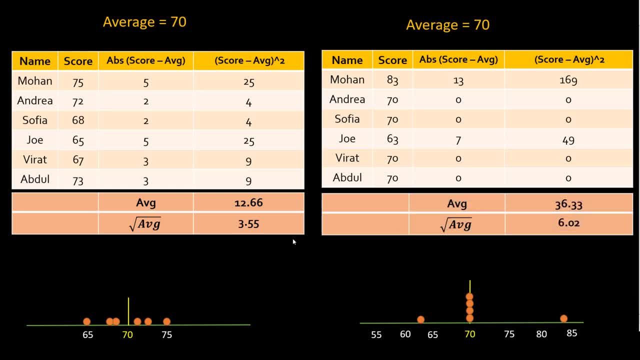 same mathematics and come up with average and square root of average. but this time I came up with 6.02. so see, here the number is 3.55, here the number is 6.02, so higher the number. and this means that the data points are spread out more, they are more widely spread out. 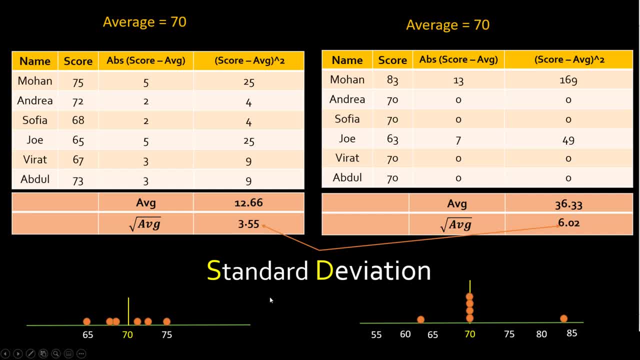 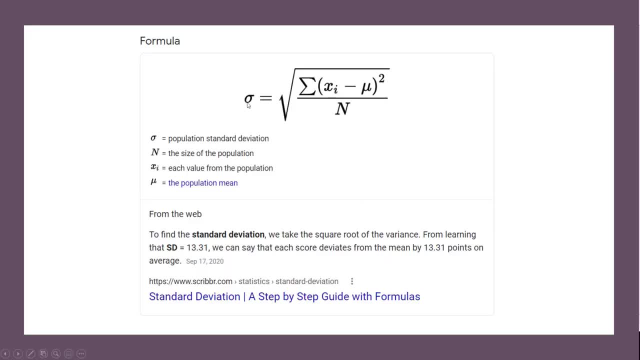 This square root is called standard deviation. Standard deviation is nothing, but you take individual data points. so here this, this particular symbol is called Sigma and Sigma is your standard deviation, and standard deviation is nothing. but you take individual data point which is minus mu is average. then you take square of individual data points, then this symbol means: 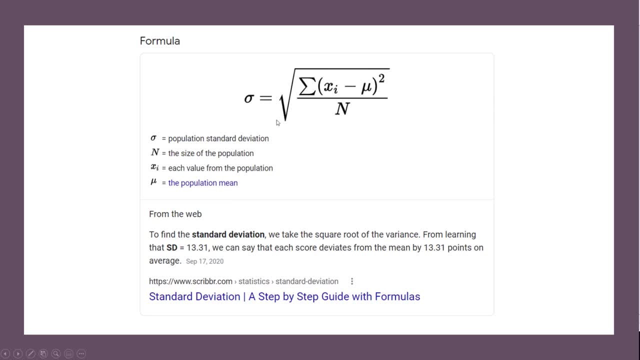 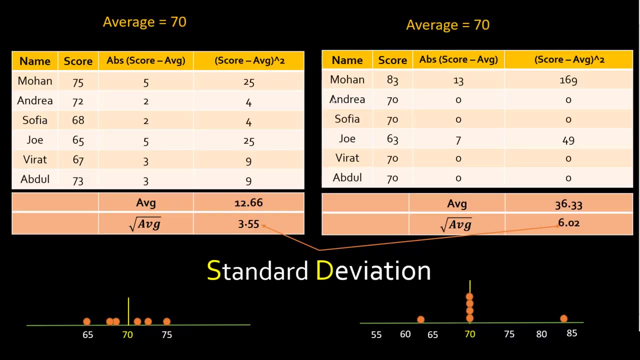 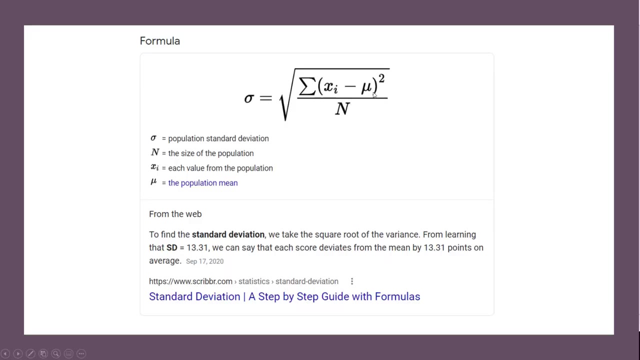 you sum it up, then you take the average and then you take the square root. see, this is not complicated, friends. we already did this math. if you look at this, this is exactly what we did, so we took the difference first. okay, so that difference is xi minus u. so that is this particular. 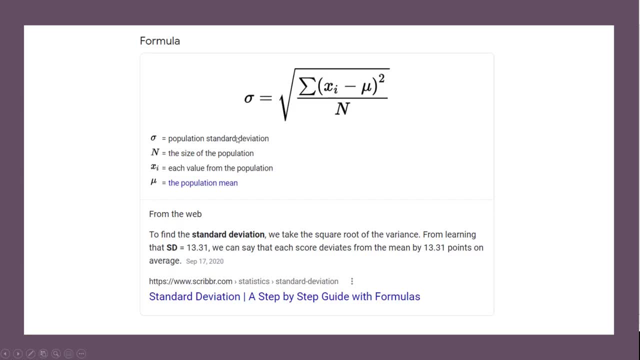 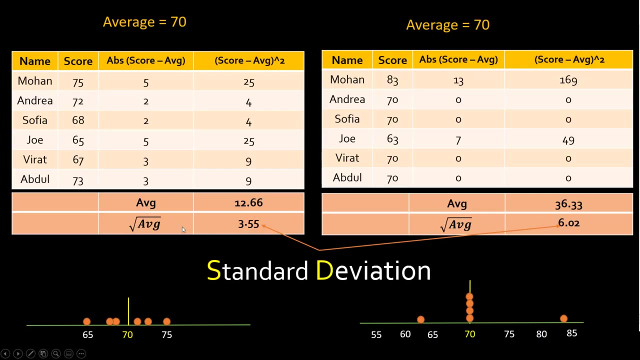 column. then we took a square of that. okay, so that is the square. then sum, sum and then divide by n- n is number of data points, which is an average. so that is this average. and then we took the square root, which is this square root, and hence you got 3.55 versus 6.02. so standard deviation is something. 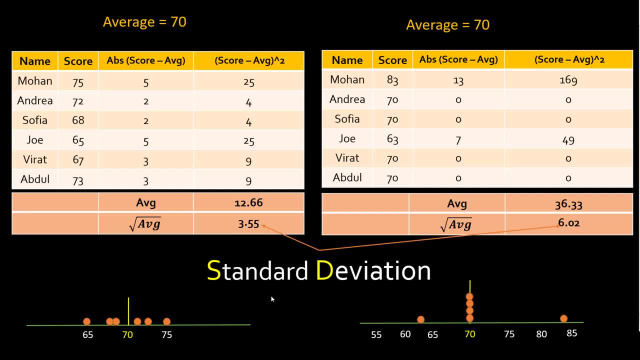 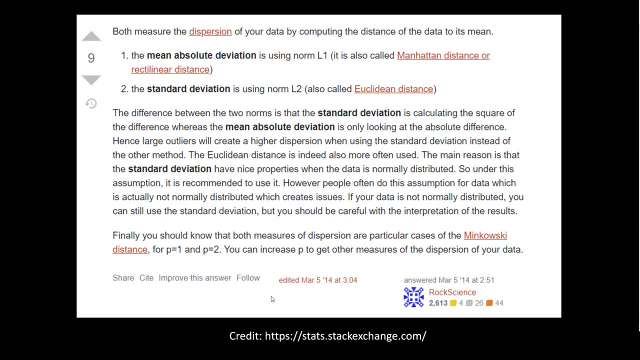 you will use a lot in data science, machine learning, statistics. these are: these are the very, very basic concepts that you need to know when you are learning statistics or data science. you might have heard about this term: l1 and l2 norm. if you're doing machine learning, let's say: 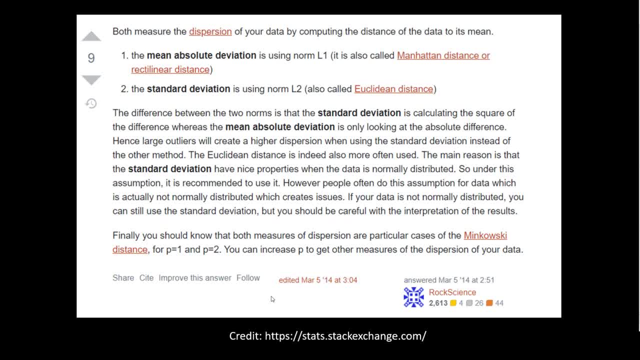 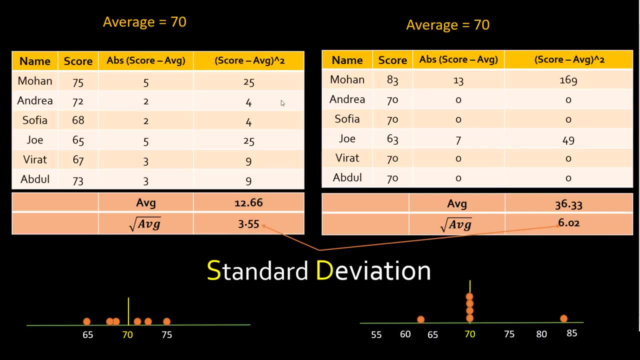 linear regression. you might have done ridge regression and lasso regression. so those are l1 and l2. l1 usually refers to mean absolute deviation and l2 refers to the standard day deviation. so we'll be using this standard deviation in future videos as well. my next: 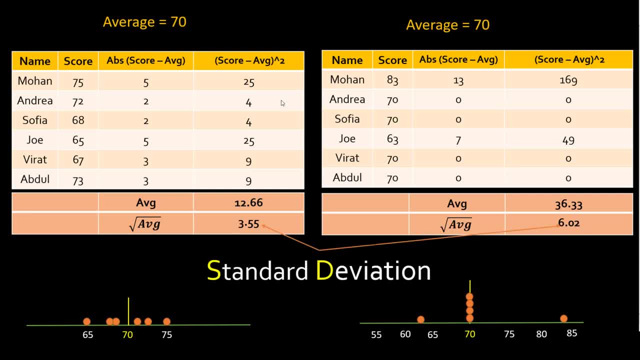 video is going to be most likely on normal distribution, so I hope this video gave you some basic understanding of standard deviation and mean absolute deviation. if you like this video, please give it a thumbs up, share it with your friends and I will see you in another next video. thank you.